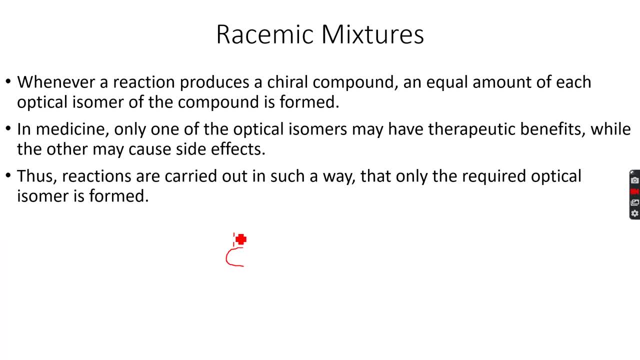 A chiral center is a carbonyl. A chiral center is a carbon atom that is attached to four different groups. So this A, then we have a, B, a, C, a, D. So this is just a wedge and the other one is a dash and the other two are the normal bonds. 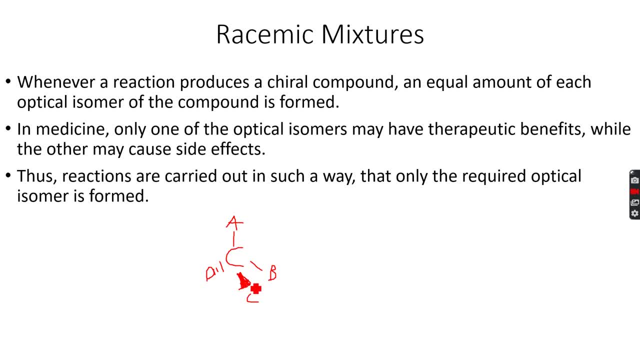 So that's how we draw a three-dimensional structure. and so you know that this is a chiral molecule because it's attached to the carbon atom is chiral Because it's attached to four different groups. So we will get optical isomers. We always get two optical isomers for one chiral atom. 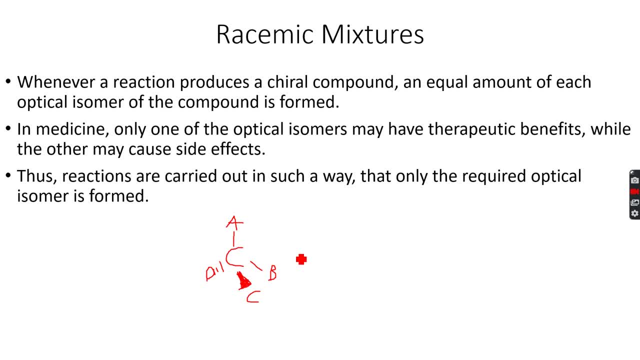 So whenever a chiral compound is formed in a reaction, then we will get two optical isomers. So we get 50% of one isomer. That means half of the product is the D isomer and half of the product is the L isomer. 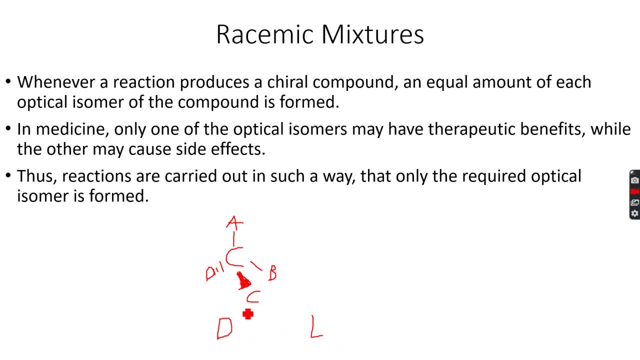 And these are non-superimposable mirror images, as you know about optical isomers. So they are produced in a 50%, 50% ratio, So one is to one ratio, and these are. therefore they are called racemic mixtures. Okay, so these are called racemic mixtures. So in medicinal chemistry, if an optical isomer is used to treat a disease, 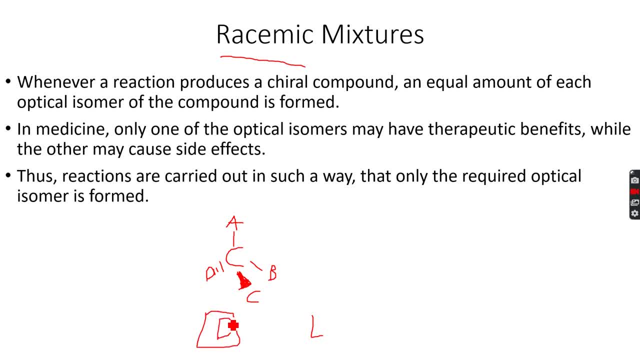 So let's just say that the D isomer is used to treat a condition or a disease, then it's not possible that we also use the L isomer, because only one isomer has therapeutic benefits. That means only one of these isomers, In this case D, can cure the disease. so if we use L, then maybe the disease will get cured, but the chances of getting side effects are higher. 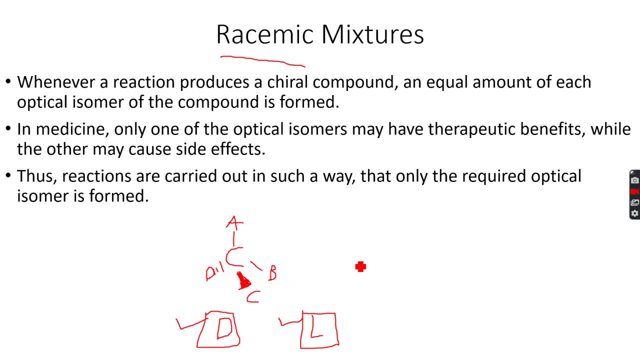 So we use the D isomer, We only use one of the optical isomers. so the reaction which produces both these isomers, it's carried out in such a way that, instead of getting a mixture of both, we get only one, because we have to use only one. 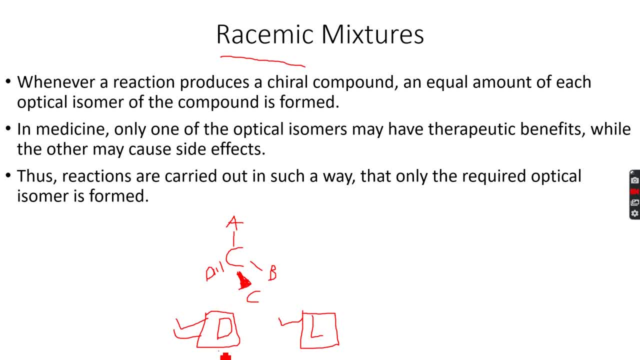 If we get a mixture and we put the mixture in a medicine, then there will be some amount of D and some amount of L. So we carry out a reaction in such a way that we only get one isomer, which is the D isomer in this case.